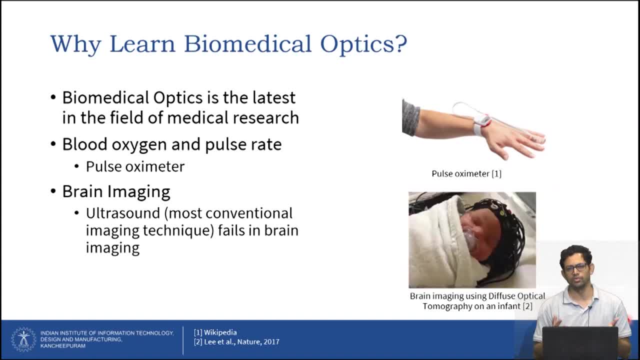 One more use of the biomedical optics is the imaging of the brain. So the brain is a very tricky place to image. For example, it has a very thick bones, So imaging within the bones is kind of very, very difficult. So people are coming up with near infrared spectroscopy tools. 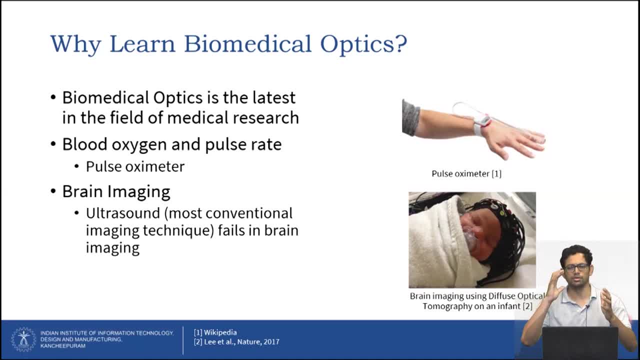 which can actually measure the size of the bone And you can actually put on top of the surface of the brain and you can actually use multiple optical fibers, as you can see on the screen on the right hand side, And you can actually image the full structure of the brain and the specific topic which is known as functional near infrared spectroscopy, that it understands the functioning of the brain as well. 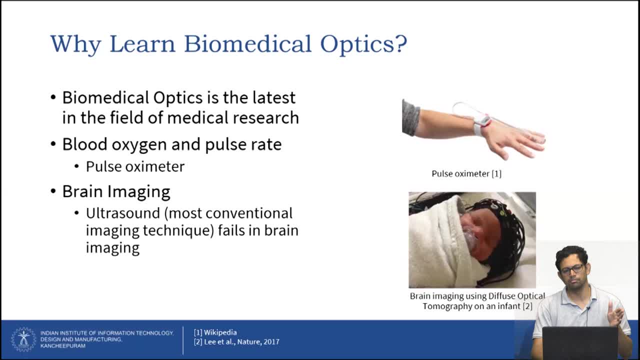 So presently the technique that may be used could have been ultrasound, but ultrasound is not that specific to detect the ultrasound waves through the thick bone, So optics is kind of being pushed as a technology that could be used within the Phoenix per se. 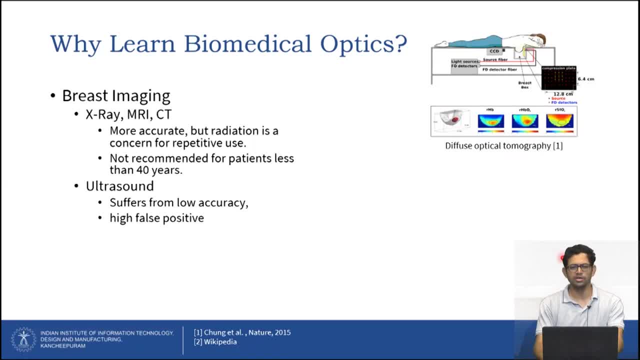 The next is imaging of the breast. So imaging of the breast: presently it is done by X-ray, MRI or CT, But X-ray is not possible. It is not recommended for people for less than 40 years and it's kind of an issue with the dense breast. 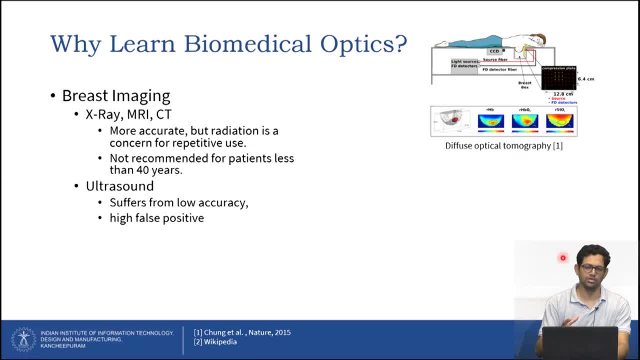 Ultrasound is another technique that people use to image the breast, but it suffers from lower accuracy and high false positive. So people are coming up with the diffuse optical imaging technique, where they actually build a system around the breast and then they image the whole breast. 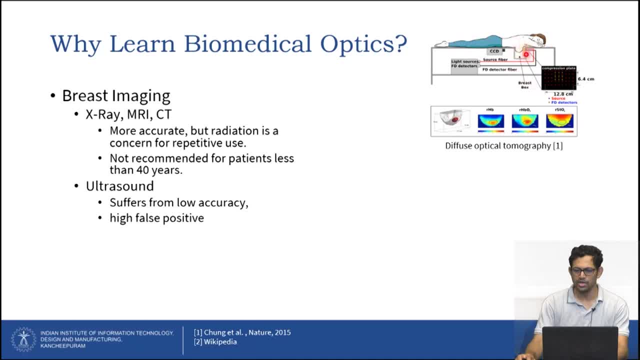 As you can see on the right hand side, a woman actually is lying in a prone position And the breast actually is not in a prone position. So the breast is not in a prone position. So the breast is not in a prone position. 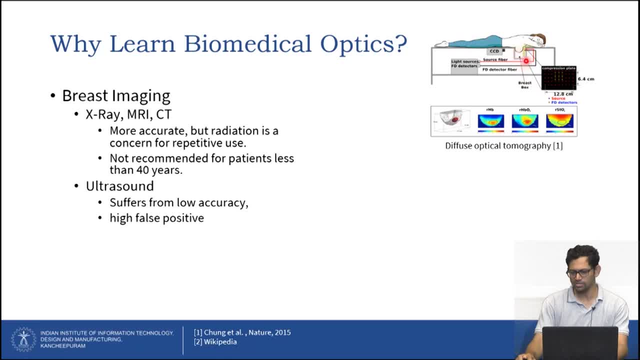 So the breast actually goes inside a box. that is in this paper by Shuang et al. It is mentioned as a breast box and it's connected to a source, multiple sources and fibers through fibers and detectors along with the fibers, And it goes to the source and detection circuit and you can actually image the whole breast. 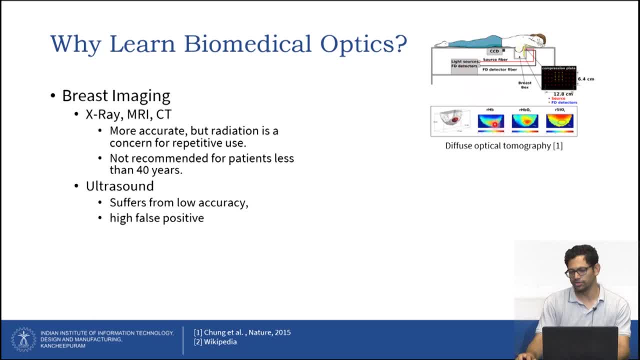 What you actually see is the hemoglobin concentration and there is all other concentration of the breast. You can actually see that- the hemoglobin concentration, and there's all other concentration of the breast that you can actually imagine the whole breast. You can actually imagine the whole breast. 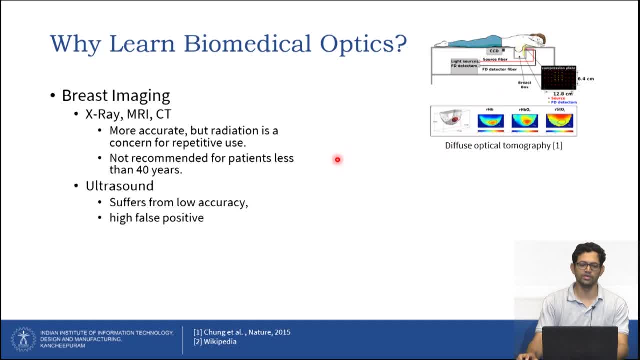 the breast tissue, constituents of the breast, for example. you have the water constituents, you have the lipid concentration, your collagen concentration. so all this concentration you can actually image. another place where optics is coming into the kind of a front is the cancer margin assessment. now, for example, a woman, as you can see on the screen, is undergoing breast conservation surgery. 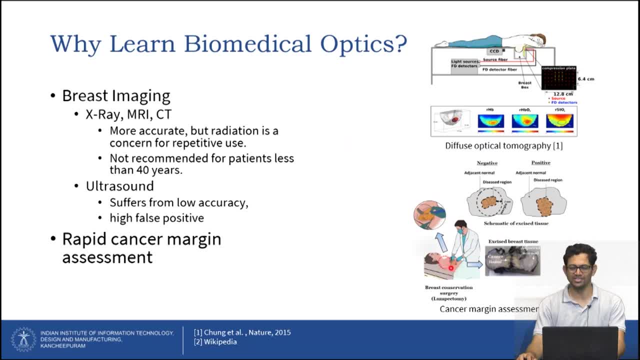 in that case a part of the breast which is kind of diseased is removed, as you can see over here, and not only the disease region but along with the disease region and just a normal region also needs to be removed. otherwise, if the, the excised breast tissue is not having 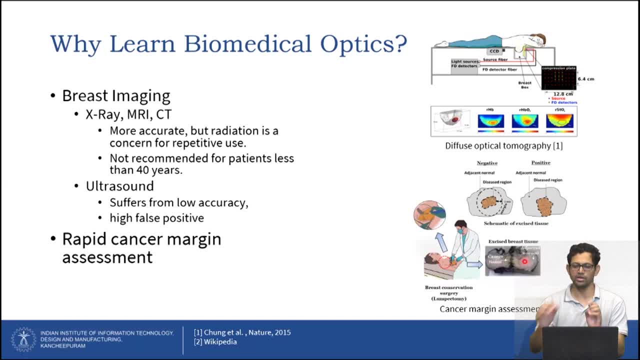 any normal tissue on the surrounding, for example. example, it is having a cancerous tissue, as you can see over here, on the periphery of the excess tissue. that means that some of some part of the disease tissue might be present inside the breast of the patient, which could lead to the reoccurrence of 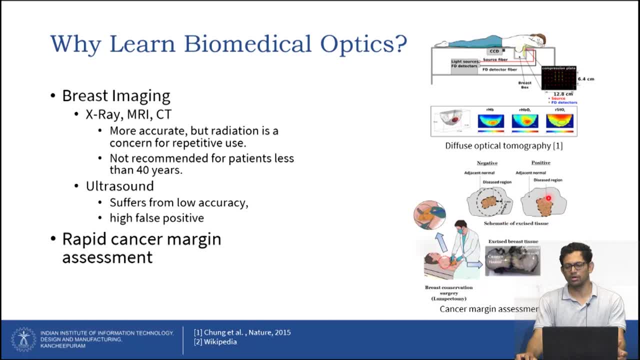 the cancer. so this is not the case that we uh is. this is kind of not desirable, right? so you kind of always require a margin, that you see over here with the dashed line of around one to two mm. that is an extra normal tissue that one has to remove, uh, and that kind of. 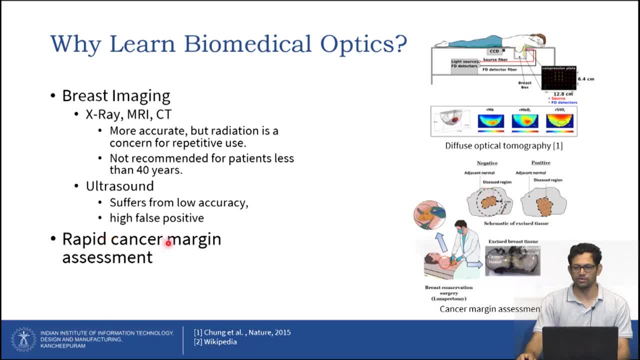 assessment is known as cancer margin assessment or tumor margin assessment. so optics is becoming a tool where you can actually understand or you can quantify on the periphery of the tissue that all the peripheral tissues are actually normal or not. okay, so that is one of the techniques that people are using. uh, next, where? 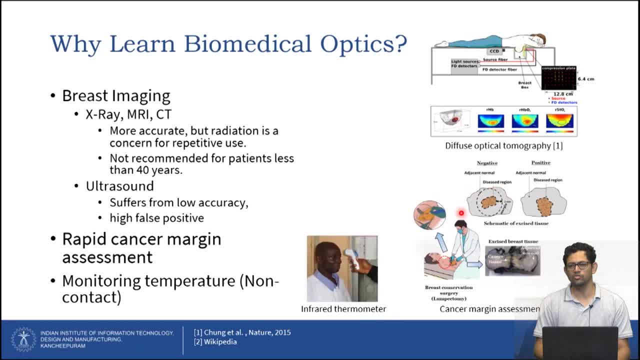 people are using biomedical optics is monitoring temperature. and this is again you would have used, you have used or you've gone through this uh during the uh the covid 19 epidemic, that uh touching using the mercury based thermometer was kind of not recommended because it it conduct it actually had a physical contact, but people were starting to use. 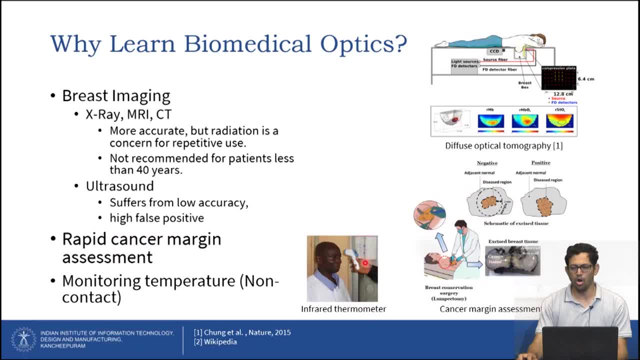 thermometer- infrared thermometer- which works on uh optics based modality and it is a non-contact base so you can easily perform multiple measurements of different different patients without actually touching it right. so that is one of the best advantage of biomedical optics: it is kind of non-contact modality. 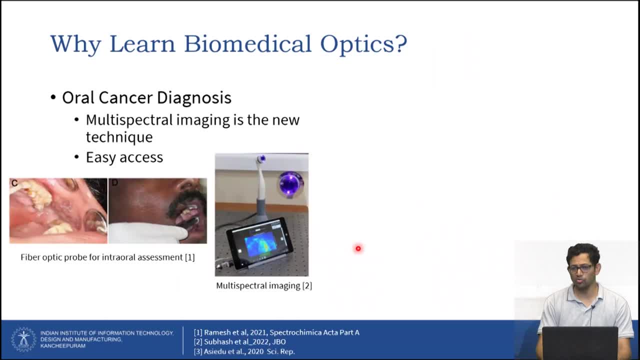 another mod. another avenue where optics could be used is oral cancer diagnosis. so in the case of oral cancer diagnosis presently, the clinician uh opens the mouth of the patient and this visualizes what are the changes or abnormalities within the tissue of the internal cavities. uh, it's kind of very challenging to uh means. 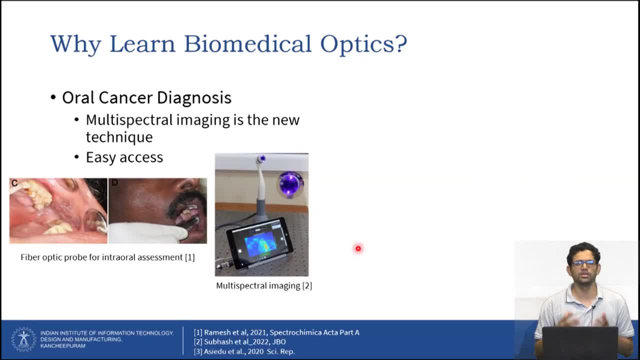 presently in the in the clinician who is specifically working in a government uh settings they are, they have to work like continuously for six to seven hours. it becomes very challenging for them to uh work with the same or continued activities of the patient accuracy right. so in such case what happens is that it becomes difficult after five to seven. 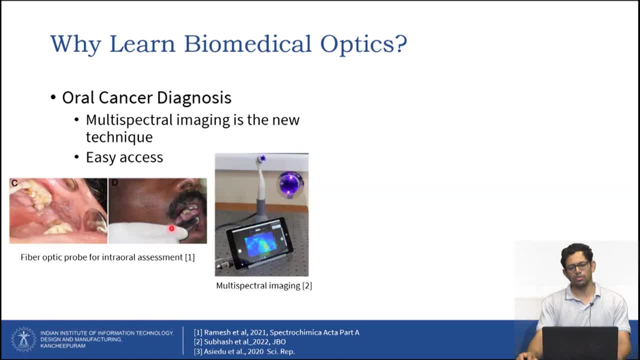 hours or so. so people are coming with up with optical based techniques to image the intraoral cavities of the tissues, oral tissues. so, for example, one of the technique is using multi-spectral imaging, that is, you shine the light using different, different light sources. for example, uh, you first shine the light with the green color, then you shine the light with orange. 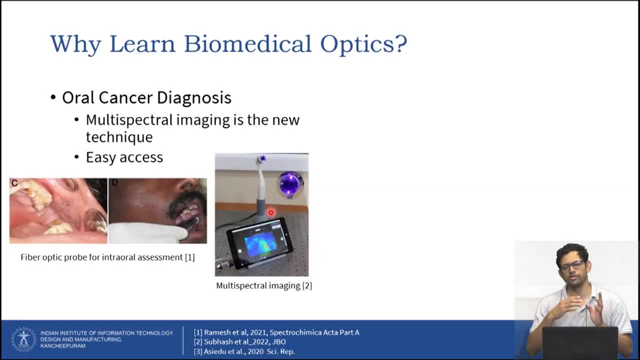 color, then you shine the light with yellow color, and then you shine the light with the red color, and then you shine the light with the blue color. so these are the separate, separate images that you have now, five, six images that you have now, and then: uh, based upon the absorption peak of 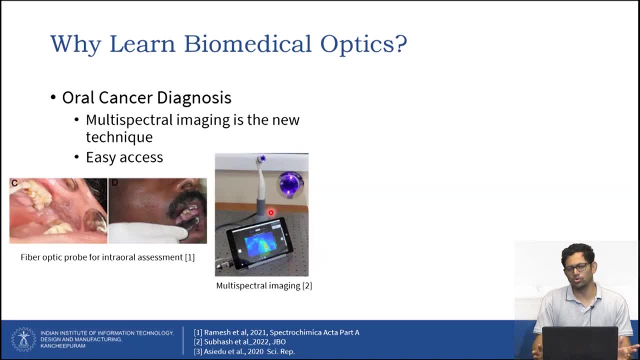 specific cancer biomarkers, for example hemoglobin, that you want to uh quantify uh the. the peak of the hemoglobin, oxygenated hemoglobin, comes around 545 and 575, that is the uh green and the yellow color respectively. so you can actually uh differentiate if the tissue has 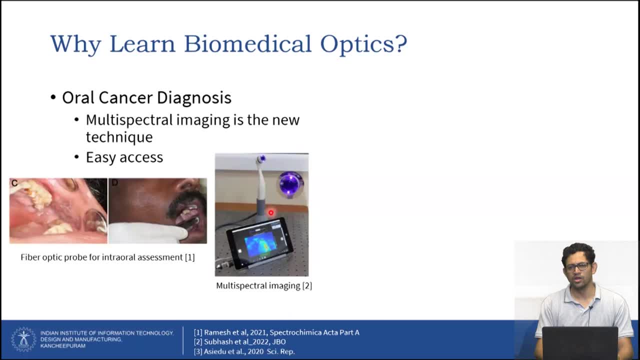 higher hemoglobin or lower hemoglobin. now what happens in the cancer is that because of the heme cycle production, there is a kind of, because of the uh, a particular enzyme known as ferrocellite enzyme, uh, the production of him reduces in the case of cancer. so in the tissues which is affected 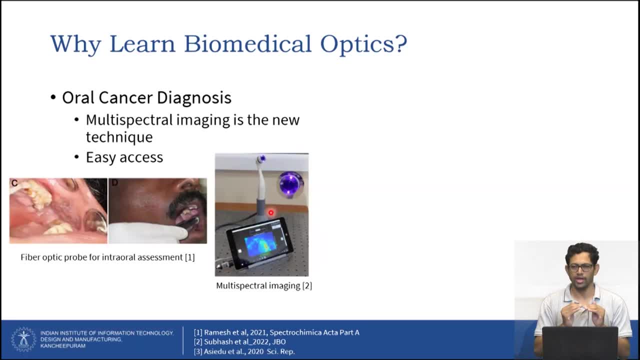 by cancer the hemoglobin is kind of lower as compared to the uh normal tissues which is surrounding the cancerous regions of the tissues. so if you try to image with a multiple spectral, multiple light source, you can nicely can see that the light which is uh coming out from a cancerous 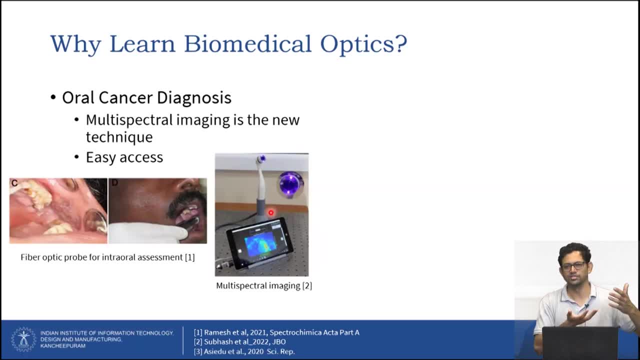 tissue is kind of starkly different as compared to the adjacent normal tissues, right, so you can actually nicely differentiate between normal and cancer. uh, the thing to know is that this is a peripheral kind of a cancerous, so it actually occurs on the surface of the tissue. 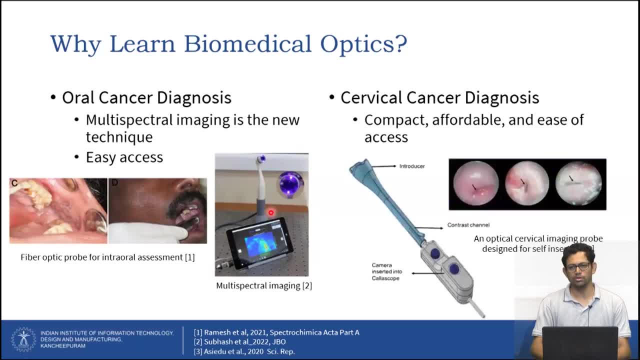 uh. one more case where the cancer occurs in the peripheral is a cervical cancer, uh, cervical cancer. so in this case what happens is that people are coming with optical modality again to uh. right now it's kind of more or more or less the work is on white light imaging, so they kind of apply a white 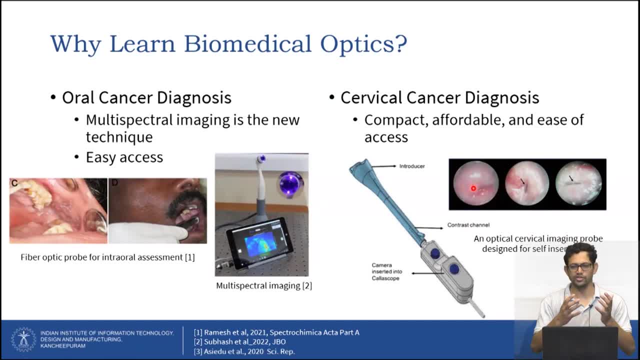 light source, which is a compound light source, onto the tissue surface and then kind of image the cervix as you can see over here and from there. uh, by applying acetic acid, what happens is that the all the protein on the surface gets denatured. now, in the case of cancerous region, what happens? 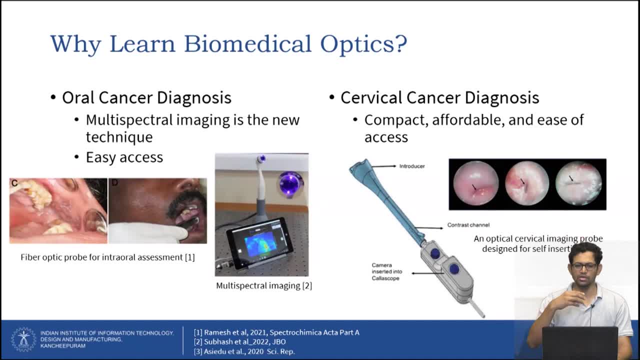 there is more protein, so uh, there's more protein which is getting denatured, so there's more protein which is getting denatured, so there's more scattering, which gives you a white color composition. so the region, which kind of white color as you can see over here, those, those are. 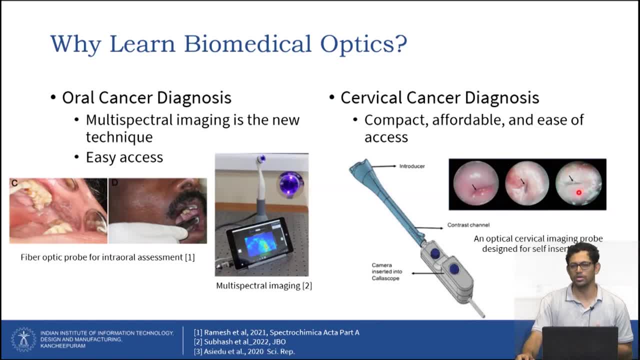 the region which are kind of affected or abnormal, or it could be cancer, for example. right, so people are specifically using colposcope- uh is the technique that uh presently used. uh again, a white light imaging modality- and then they are introducing some kind of a probe that can be uh inserted within the vagina, that is, a transvaginal probe. 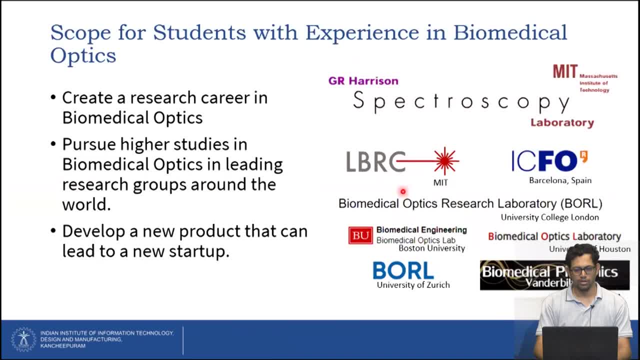 imaging probe. so so what is the scope for the students of uh after uh having the course on biomedical optics? so there's a lot of scope so you can actually have your research career in biomedical optics or medical optics. there are a lot of groups, as you can see on the right hand side. uh, you have a mit. 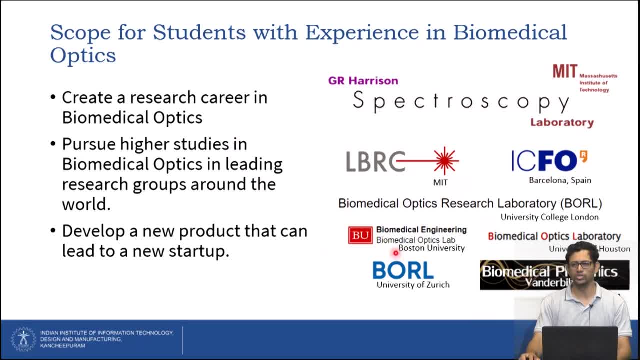 biomedical photonics in vanderbilt. so a lot of opportunities are there all over all around the world. after learning the basics of biomedical optics- so not only the research career- you can pursue higher studies. if you are right now performing your or doing your undergraduates or post graduates, you can do your higher studies as. 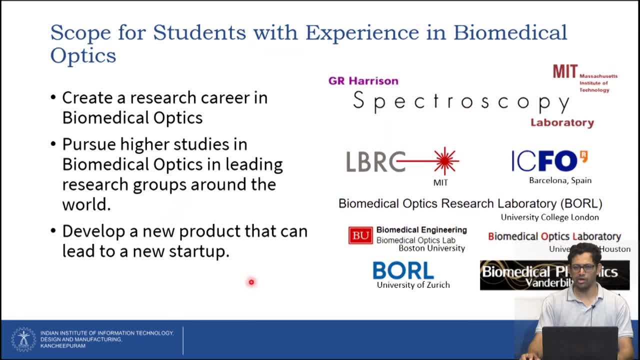 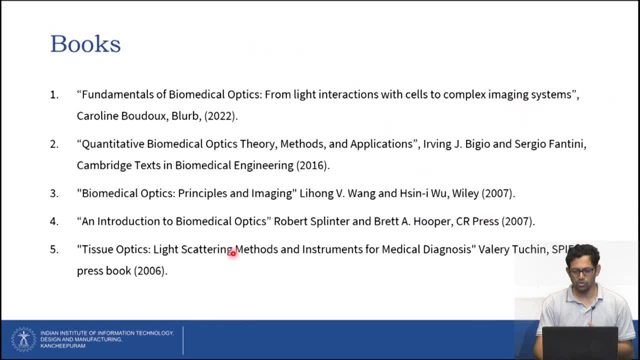 well in biomedical optics. and then you, in addition to this, you can also develop a new product which can lead to a startup. i will just go through the books now. so these are the books that we will be covering through the course. okay, so main book would be the. 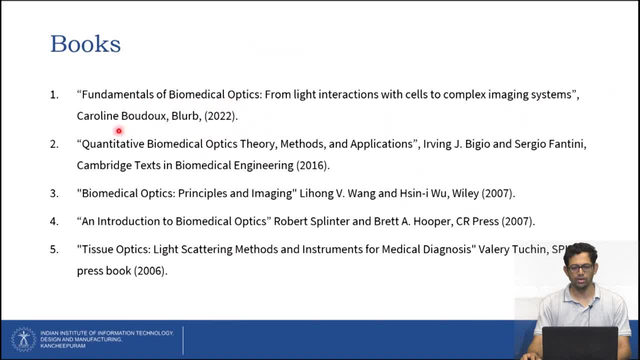 by the fundamental of biomedical optics. it's a very nice book by calorin uh borax, and one more nice book is quantitative biomedical optics: theory, medical and application by irving biggio and sergey of anthony. so these are the two main books that we will be covering throughout this course and one more good book is tissue optics. 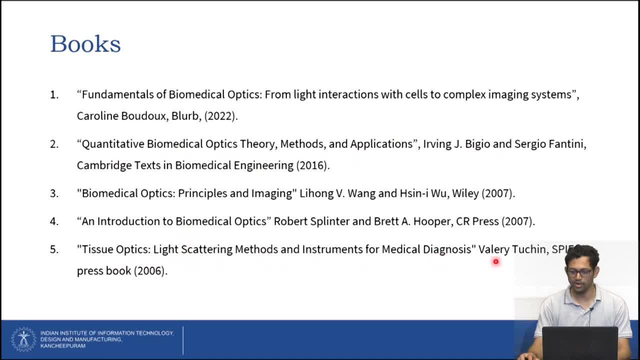 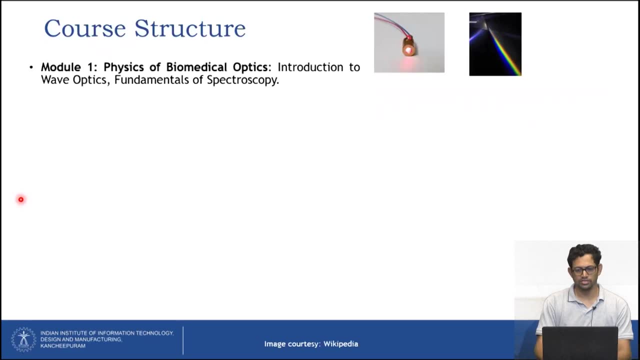 light scattering method and instrumentation from medical diagnosis by valerian tucin. the second, the third and fourth books are are kind of the legacy books that have been used, uh, thoroughly till now. so let me cover the core structure. so the core structure is the first module would be: 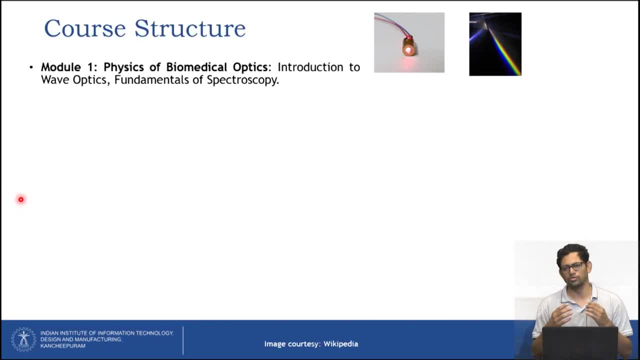 on physics of biomedical optics. so how does the light actually interacts with the tissue? for example, i i just you might have. everyone has a mobile phone right now, so i uh enable my light source, that is my torch, over here and i shine it on my, on my. 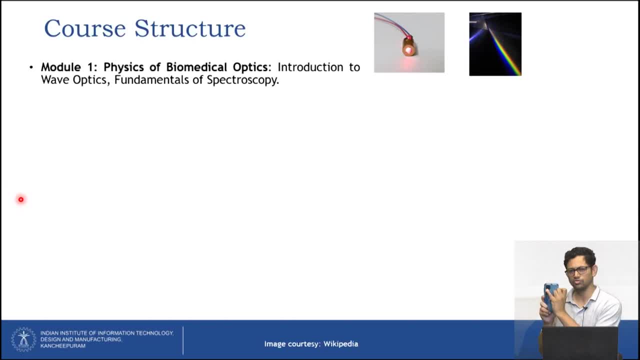 hand, on my finger. now, what can you actually see? so you, you can do this experiment with your finger as well, so you can use it your pinky finger. and what do you see? if you shine the light on your pinky finger, you actually see a red color, right? so 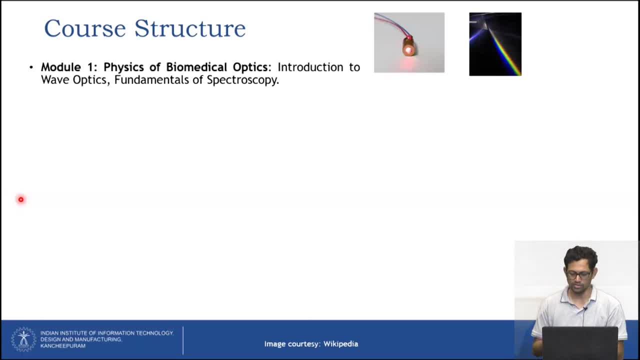 the next question that comes to your mind is: why do you actually see the red color? so this is the reason. the reasoning behind this formation of red color is what we will read or learn from this course. we'll not understand. the reason behind this formation of red color is what we will read or learn from this course will not. 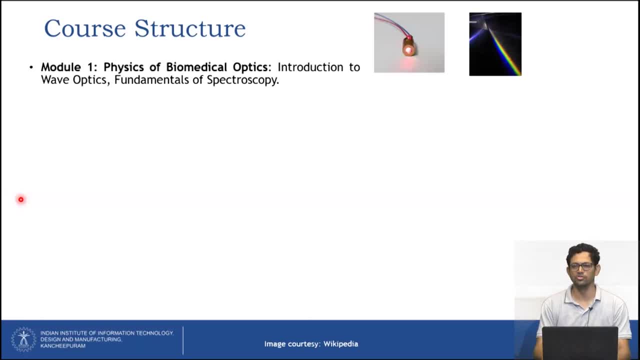 just learn about the theory, but we'll also do few experiments which could help you to understand and appreciate biomedical optics. next we'll talk about the theory. so the light which propagates through the tissue, so it undergoes two basic physical principles: that is scattering, that is, how much light is being scattered away. 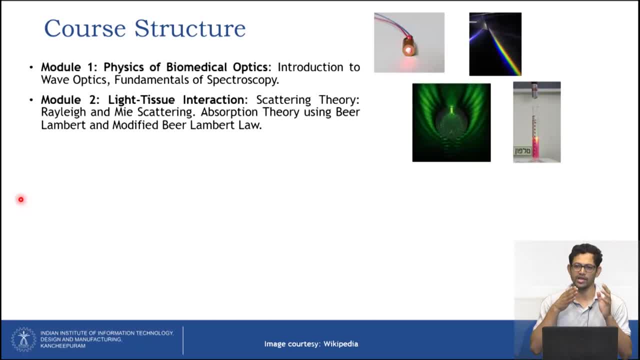 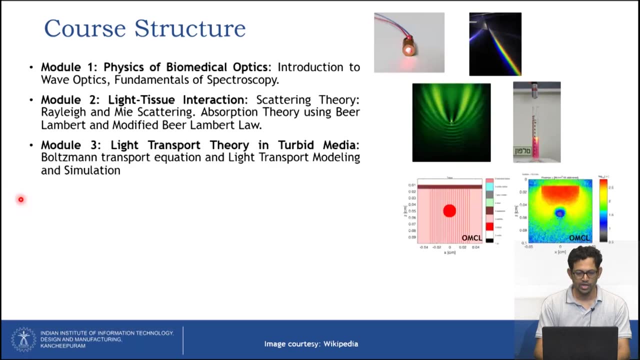 and second is absorption. so how much is the light being absorbed as it passes through the tissue? okay, so in absorption, we'll learn about beard lambert law, modifiedly, beard lambert law. in scattering, we learn about rayleigh scattering and my scattering. next we'll talk about light transport theory in turbid media. 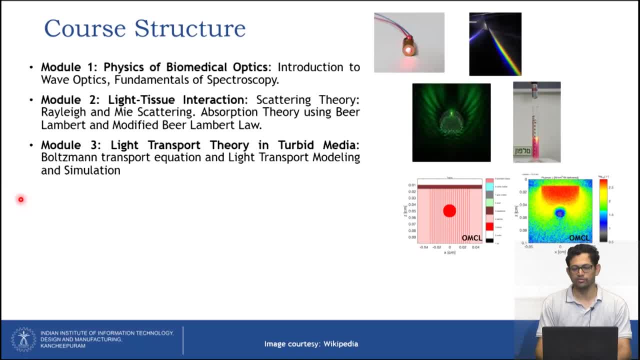 so that is the boltzmann transport equation, and then we'll apply some kind of approximation to decrease the complexity of the equation because it's kind of very complicated to solve. another way is to solve is using a monticle approach. is what we also will give a demonstration on. 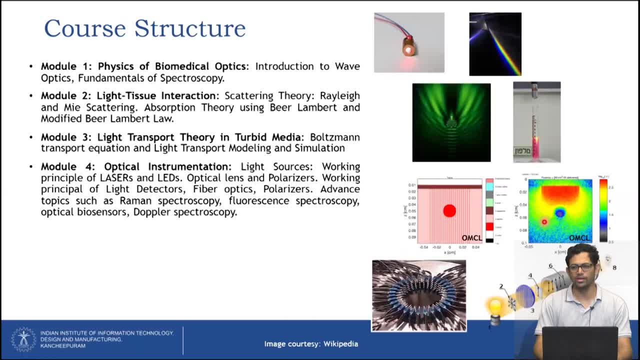 then we come to the one of the major component of the course is optical instrumentation. so we'll talk about how to work with lasers, how to work with leds, how to drive particularly the lasers and leds, how to drive the detectors. then there are a lot of optical systems. 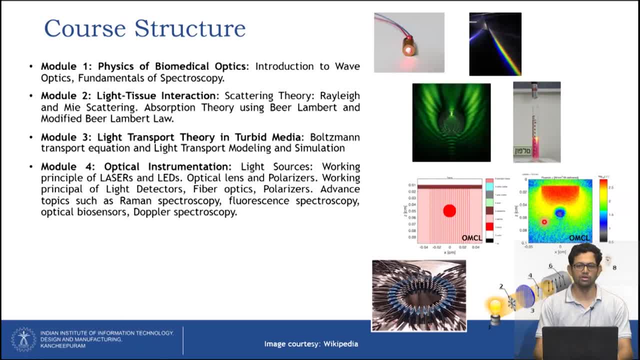 such as filters and polarizers. so we learn about those things in detail and then we'll talk about advanced topics such as diffuse reflectance spectroscopy. we'll talk about raman spectroscopy, fluorescent spectroscopy, optical biosensors and doppler spectroscopy, and the final module would be on. 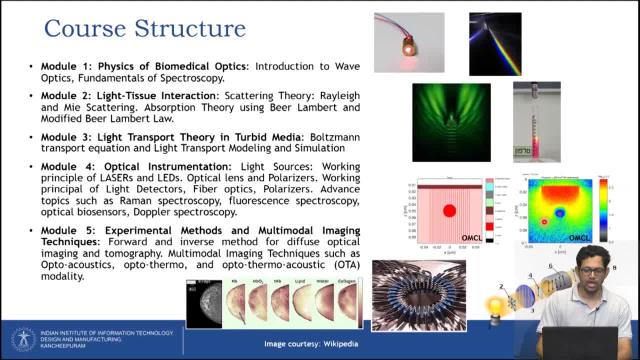 experimental methods, so we'll do few of the lab experiments- and then multimodal imaging, so we'll see uh techniques where along with optics you can actually take uh acoustics, for example, so you can merge two different fields and then you can try to see how you can.